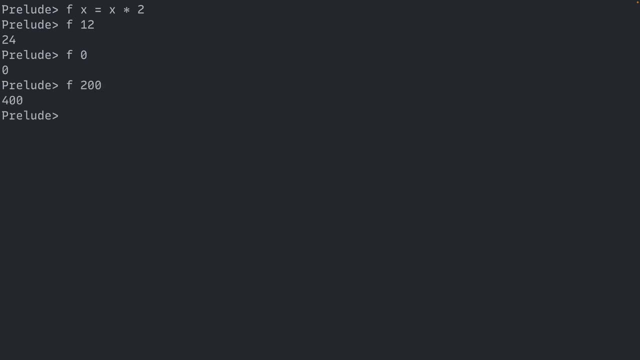 f, that will give you 400.. As you can see, it's kind of like any other language, But the key part to notice is that these functions are what we call peered, So they are deterministic. They do not access nor modify any sort of outside data. 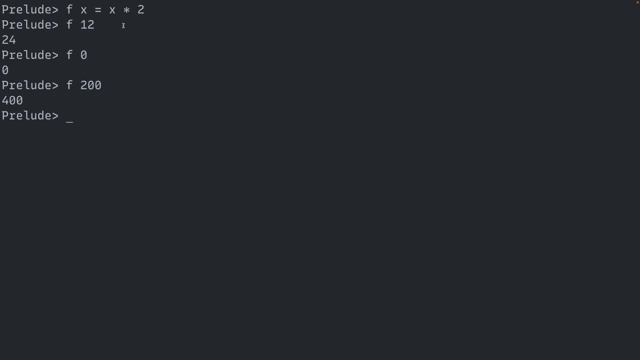 So whenever you give it the number 200, as you can see, logically it will always give you 400 and nothing else. So a great advantage of this is that, by declaring functions to be something that is to be calculated or to be expressed, rather than something to be done, 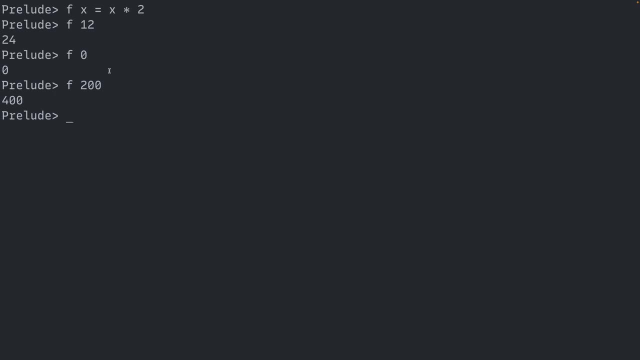 you can much easily test something, because if you were to test a function but you had to set up, for example, your app in just the correct way or else it might have a chance of crashing, that's very hard to test, But with these functions, if you give it a number, 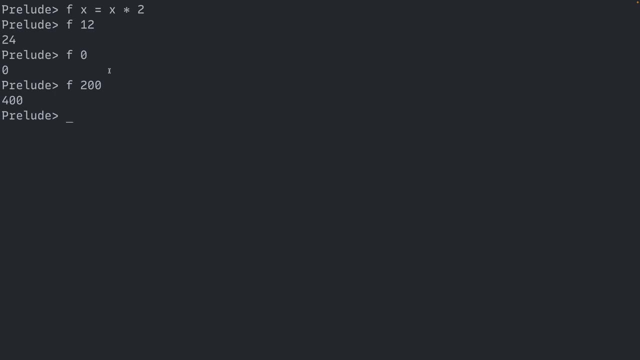 to the number you expect. you know it works. Okay, so those are functions And this is really similar to what we would expect, for example, as an error function in JavaScript. So let's say we run a Nodejs, we can just say something like: let f equals to x, error function x times 2.. 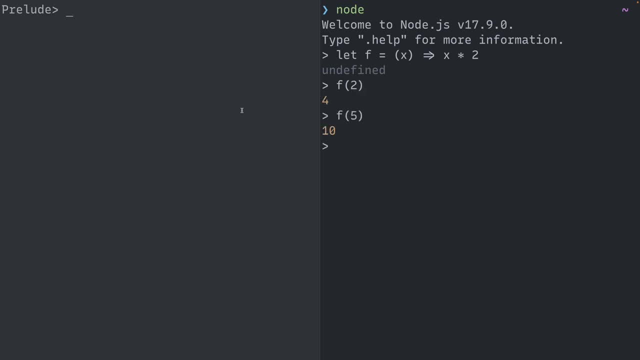 And something like this gives you like similar results And, given the nature of Haskell, it gives you a wider array of stuff. So let's say we want to make a word count option. All we can say is, for example, count String equals to length of what. 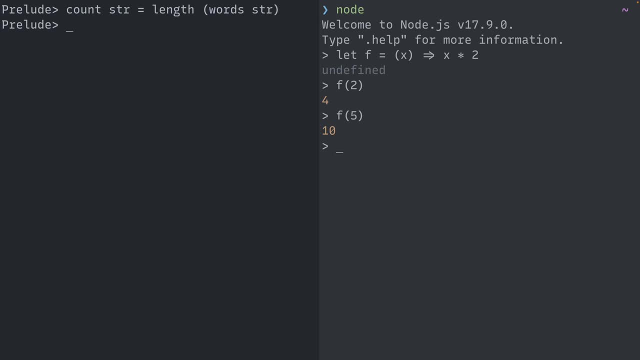 Length word string. And now we have that done, we can just say something like: count, the quick brown fox jumped over the lazy dog. Let's just write a sentence like that And that will give us 9 for each of the 9 words in the sentence. 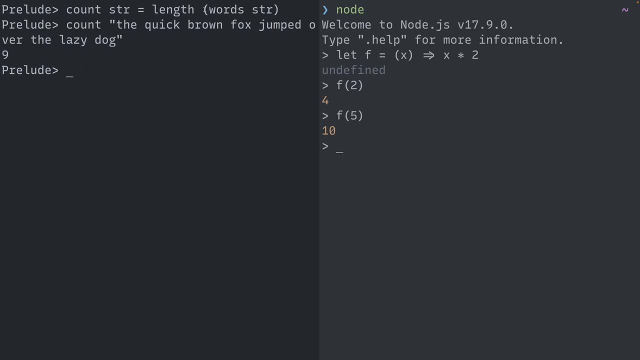 What this does is basically the word splits string into a list of smaller strings for each word as it spaces, And then length just gets the length of this. So these are really the main things that functions do. They're simply an expression that you can evaluate. 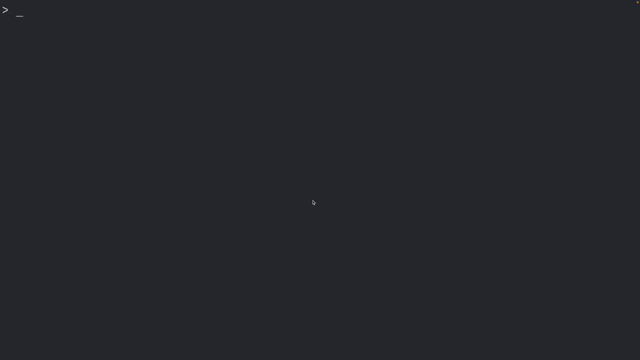 OK, now we're back in JavaScript, just to show you a quick thing. So let's say we have a function that I have already wrote called add, And we can just add two numbers by passing in a number like that. right, We can say: add 5,, I don't know 10, and it will give us 15,, like that. 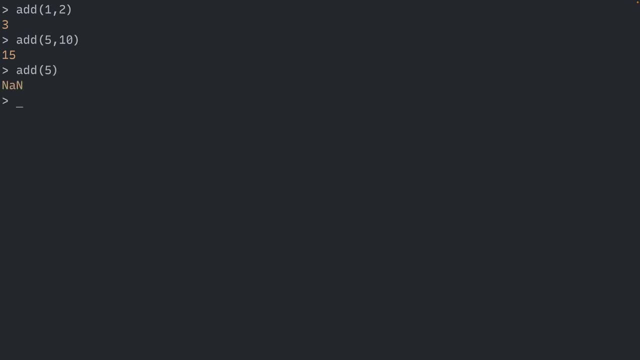 Very simple. But if we only pass it in like a variable called 5,, this will fail, And for obvious reasons, because we haven't produced enough parameters to give to the function. But what if I show you an alternative to this function? 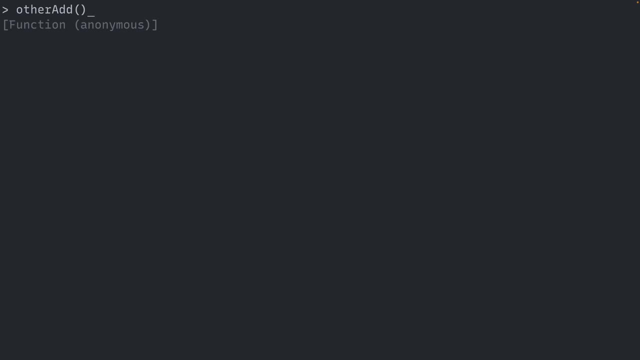 And now we have the function other add And you can see what it does. So we have 1 and then 2, like that. We have two parentheses. this time We can give it 1,, 6, like that, Or maybe let's say 10, and it will give us 16.. 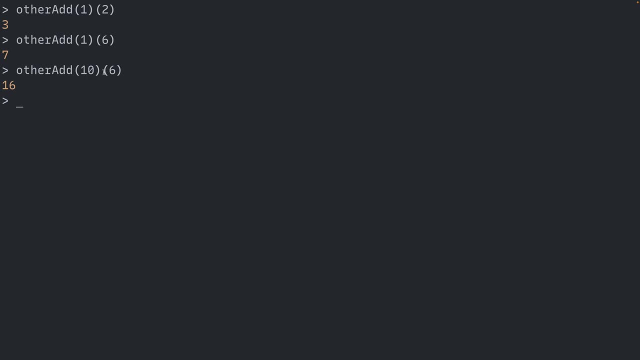 So how is this done? This is actually default stock JavaScript. Let's look at this a little bit clearly. First, we only have the function other add, which takes the number 10.. So how are we calling it again? Well, the simple answer is that we. 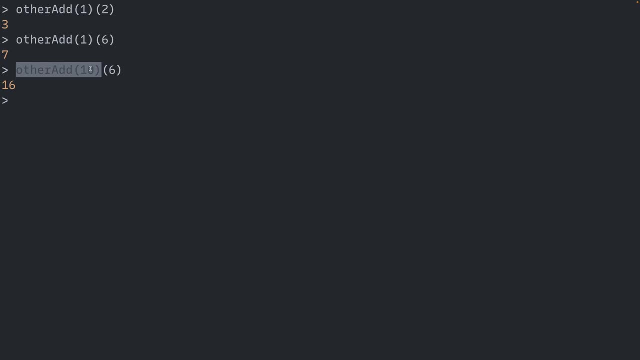 basically create this function when called that takes only one input, But it returns a new function that also takes one input. Therefore, you kind of divide it into two functions And you can only apply part of it. We can say something like: let add 5 equals to my other add. 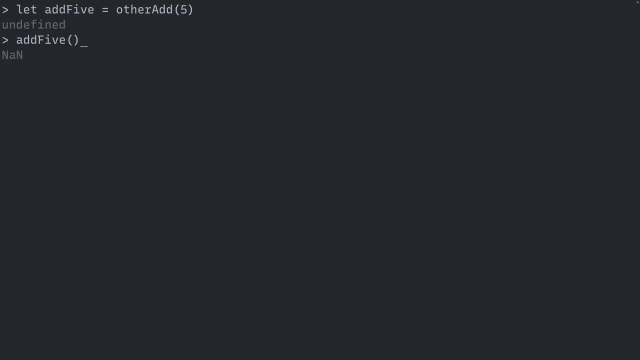 So we can just say 5. And that's it. Now we can call it add 5.. And so we call it 10, and it adds 15.. If we call 1,, it gets 6.. So you can apply part of the function. 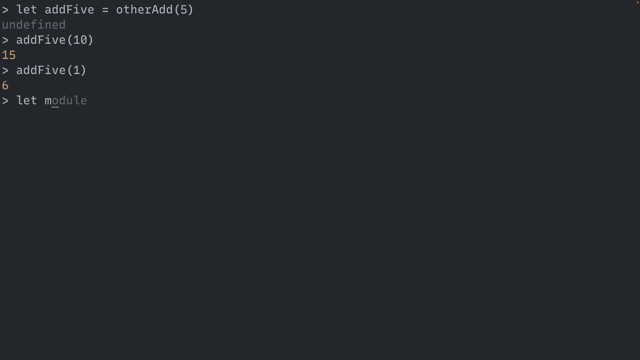 And the way we had done this is very easy. So let's say, we write my add: This is simply x, But this time you only pass an x and then you do another one, And here you do x plus y, And this double arrow may feel like some unfamiliar syntax. 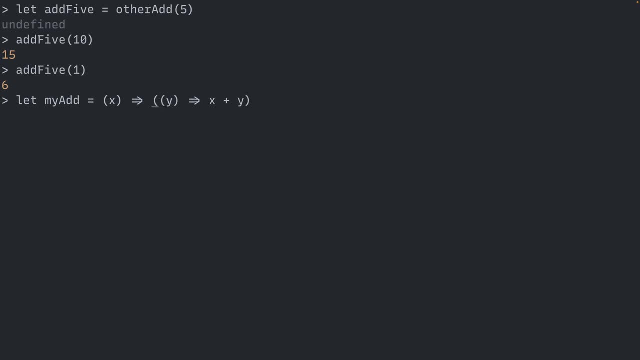 But if you look at it closely- let me add some more parentheses- you can see very clearly what is happening. You're simply having one function that returns this, another function which also takes a value, And then, because the value from x is stored from the outside function, 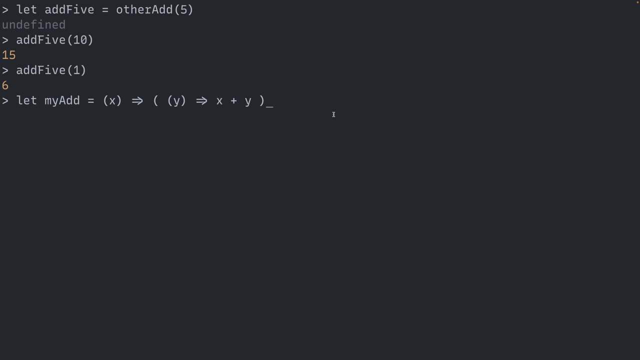 you can then use those two. if you use two parameters In Haskell, this is actually the default. So let's take a look at this. To write the same with two parameters, we simply need to say: add x. y equals to x plus y. 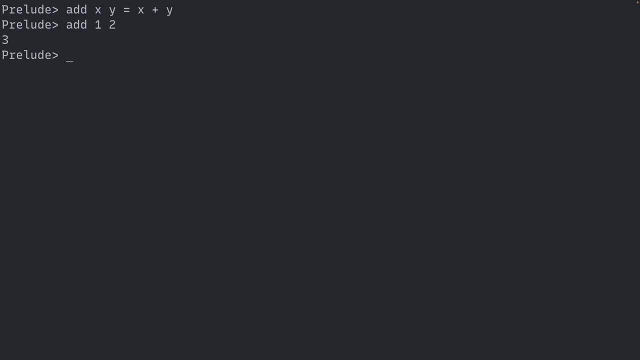 And now we have that, So we can say: add 1,, 2, and 3, and it gives the correct answer. But we can also say, for example: add 5 equals to add 5,, like that, And now we can just call add 5 as any number we want. 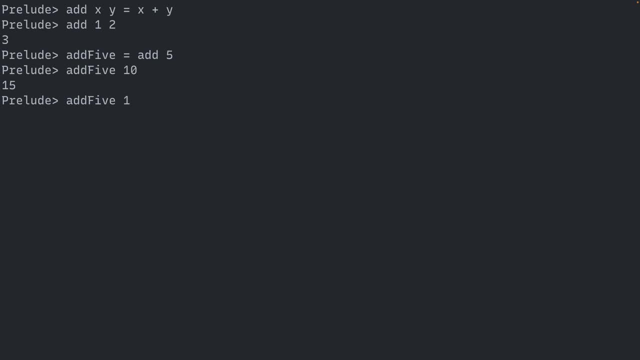 and it would do the same thing. So this method of partial application of functions is actually really, really useful. So, for example, the syntax would be a little bit unfamiliar. but we have the map function, which basically loops over a list. It goes over a list and then applies a function to every one of the values. 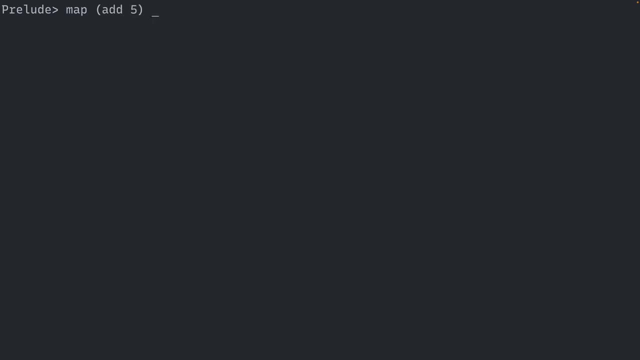 So we can say map: add 5 here, and then say 1,, 2,, 3,, 4,, 5.. And for each of these you get 6,, 7,, 8,, 9,, 10.. 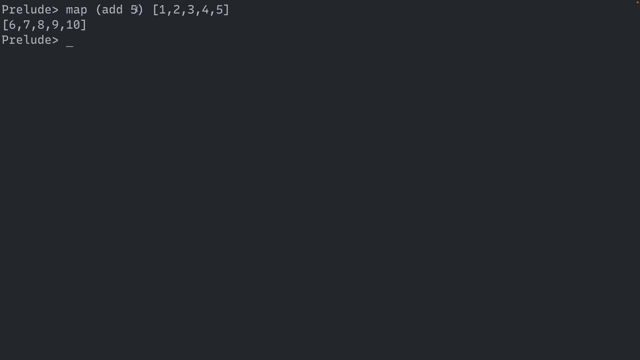 And all you had to do is just give one of the parameters to add, so that, instead of an add being a two parameter, it becomes a one parameter function that can be applied to numbers, And in fact it was never a two parameter function. 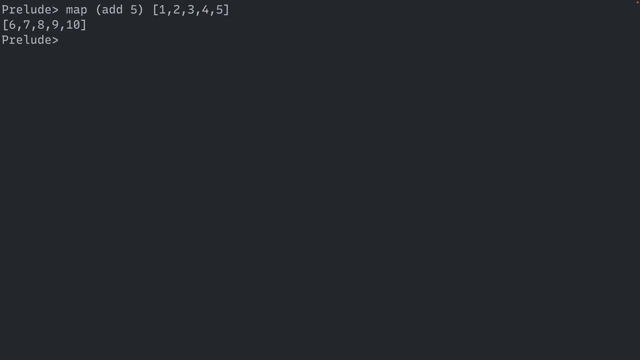 All functions in Hasco is basically essentially one parameter. So there's a command for getting the type of something and we can say type. Let's first look at add 5 to understand what it does. So this part you can't ignore. 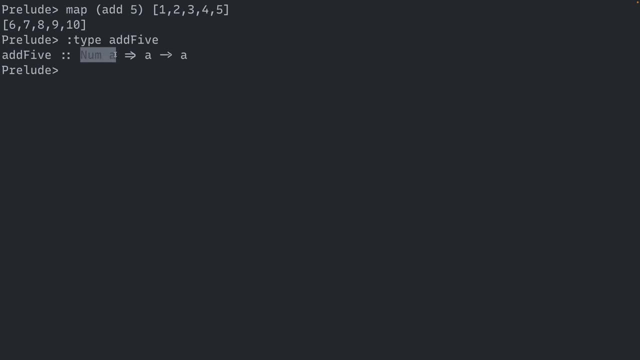 That's just a name, that just signifies type, And numA just means that this is a type where it has to be a number. But here's what we need to look at. So we have a to a, which means a type of a number to another number. 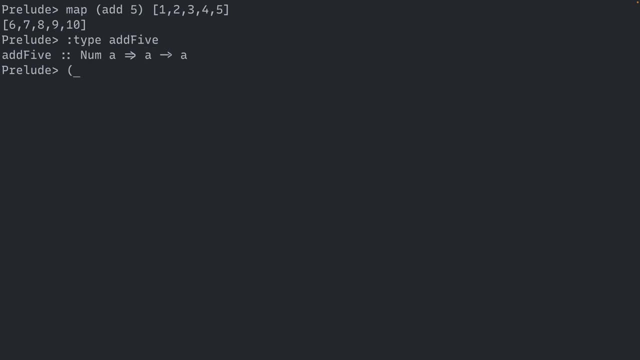 And that's exactly what addition does. All right, You would assume something like for add function. it would be like add a a to variables to 1, right, But that's not actually how it works. So let's look at type of add. 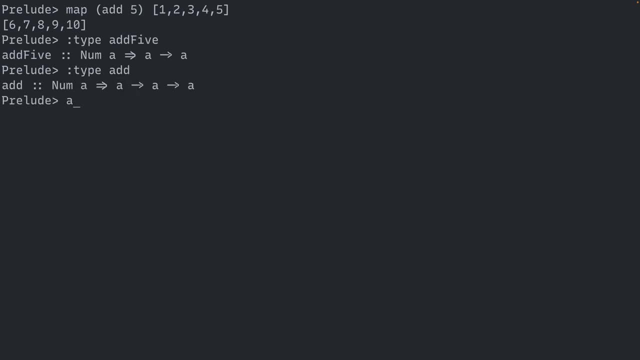 And you can see it's a to a to a. So, just as a JavaScript example, if we make this clearer, we can add some parentheses. So first, this is a one parameter. This is one function with one input, right A, which gives you another function that also takes another number. 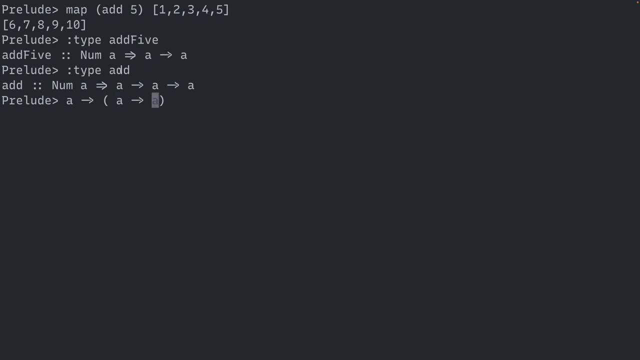 and gives you a final number, And that's how you basically have functions with multiple variables in Haskell. So partial functions aren't just for convenience, but also a pretty key part of the language itself. So, for example, instead of saying map, add 5,. 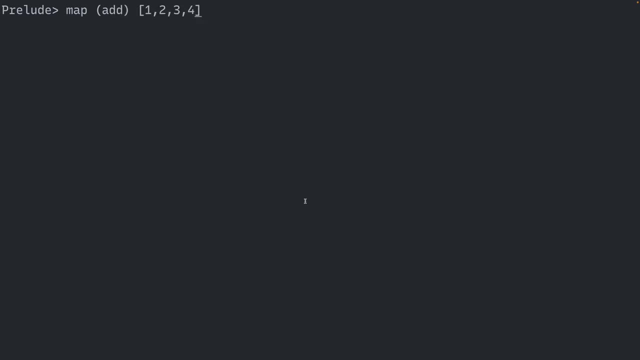 we can say something like map add. What would happen is that this is perfectly valid, despite the fact that it accepts technically what we see as 2 parameters, Because this time it's just that instead of returning a list of numbers, it will return a list of functions. 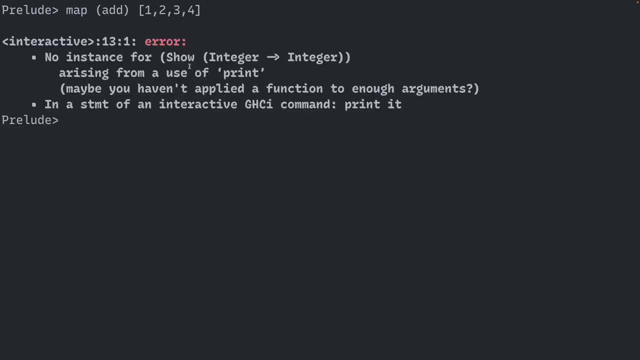 And if we press enter it will show something like an error, but that's only because it doesn't know how to show a list of functions. But this expression is perfectly valid and we can use it later on. And that's the key part about functions. 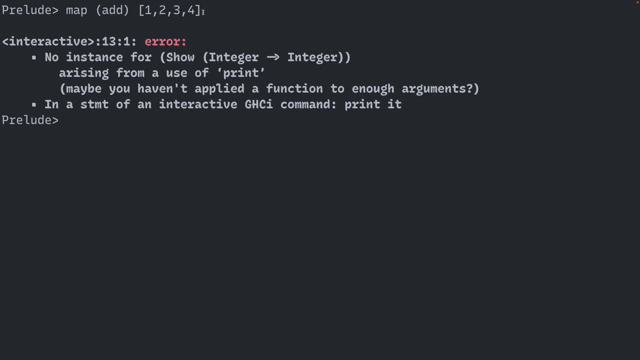 They're all the same shape, except that some functions return other functions instead of returning a value directly. Let's say we write another very easy function, like I don't know, test f. x equals to f And what this does is that it accepts a thing called f. 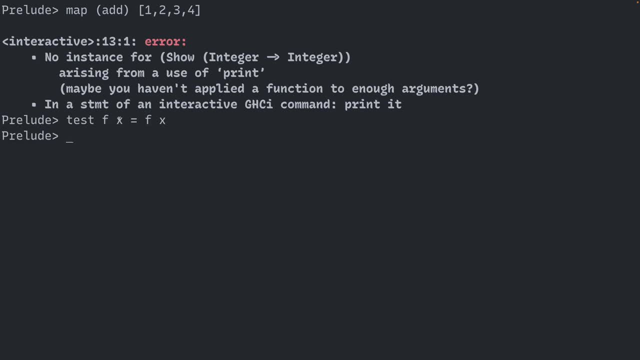 and we just call it f because to signify it's a function, and then we pass it in a value And then we actually call the function we just passed in with the value that we also passed in. So just to add the example, we can say something like: test add 5,, 10,. 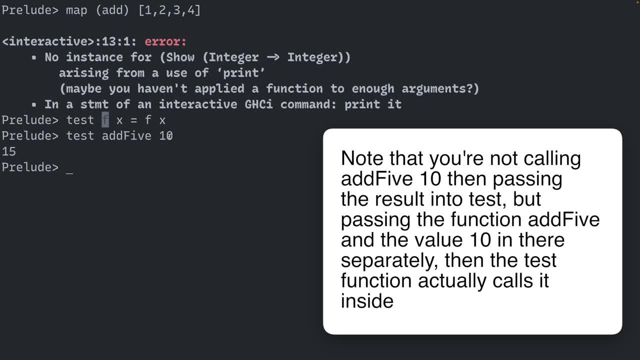 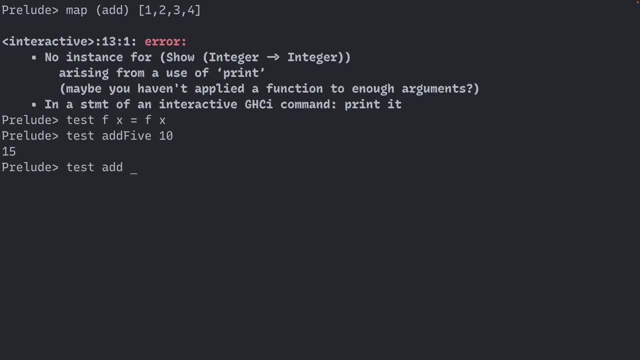 and this will give us 15.. Because f is add 5, 10 is x. add 5, 10 would be 15.. However, we can also say: test: add 1, 2.. Even though it wasn't made for it. 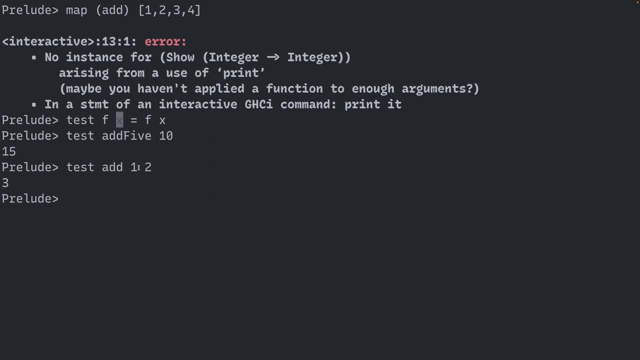 It technically only accepts the value 1.. So what happens to the 2?? How does it also work? That's because this expression gets evaluated first. This entire thing is equivalent to calling add 1.. But add 1 itself evaluates not to a value, but another function. 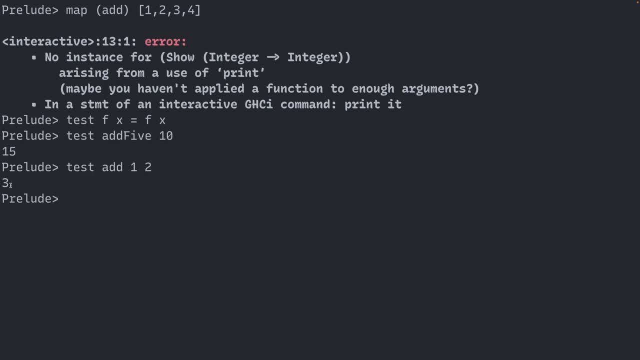 2 can also be passed into it. Therefore we get the final result of 3, despite not making the test function initially seeming to fit output with 3 numbers. So you might be looking at this and wondering how Hasco can calculate basically anything other than just pure math functions. 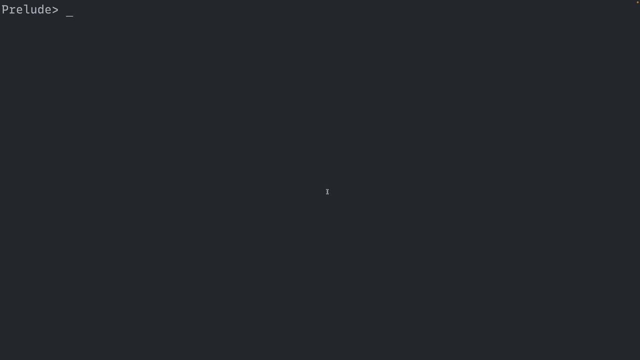 After all, everything you seem to look at has to involve state Like, for example, if you're coding a video game, you're coding a web app or anything, If you don't keep track of what's happening, how are you supposed to do anything with it? 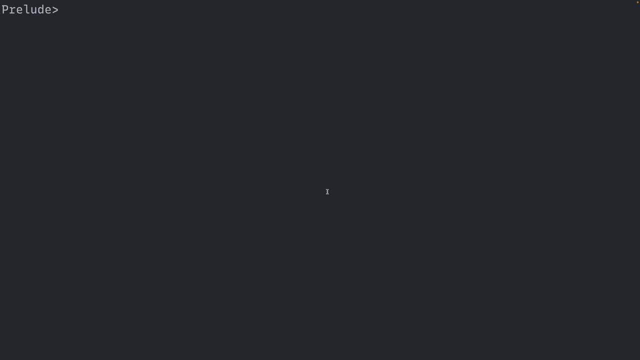 Well, that's the problem with our chain of logic, right? We tend to think of state as like a data that you keep there and then all of the functions access and change. However, in Hasco, there's actually ways to get around this. 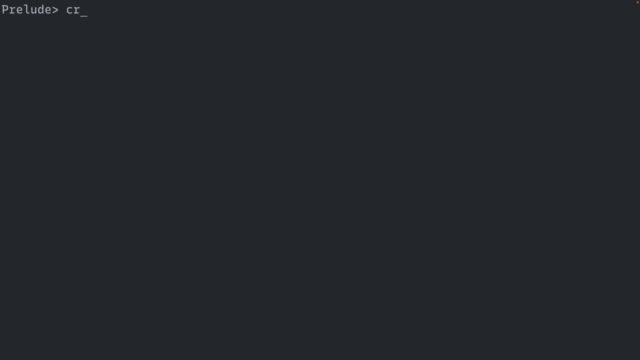 Let's say we have a video game right, You know where this object is in the player. So we can say something like: instead of saying, for example, world equals to create world, player equals to create player, player dot move upwards. you can simply say something like: create player right. 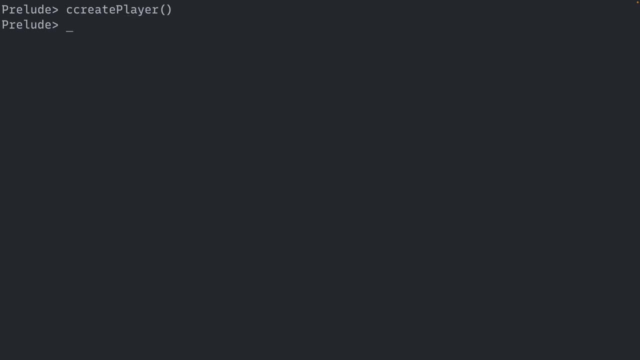 First of all, and that returns the player. And then what you do is that you have a function that wraps around it, that says, for example, move up, and that accepts create player like that, And then you can. of course, this isn't actual Hasco code. 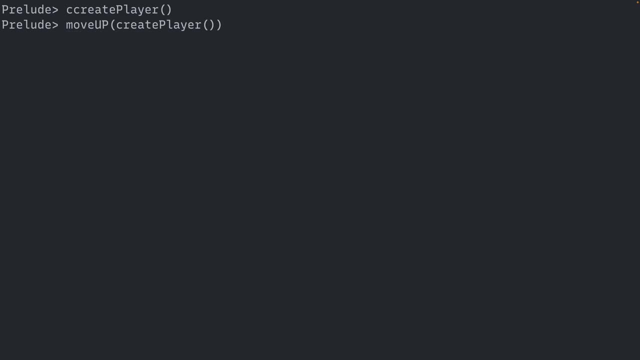 You won't have parentheses and anything else. And then you have another one that's like I don't know take damage, and that you wrap it around. So each time the value of the player is actually moved from one function to the other function, 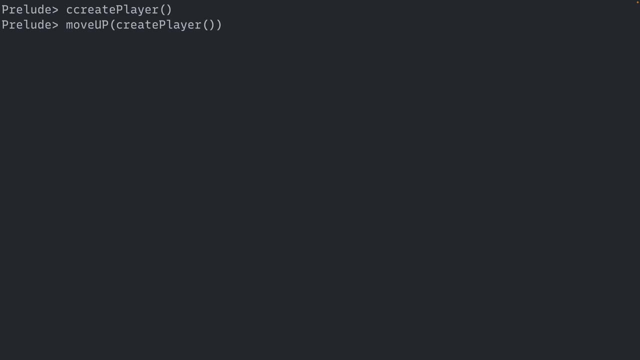 And you can see that data can flow this way as well, without ever changing the initial player. that was created, so that none of the functions that, for example, are referencing the original player would ever get affected by anything else. Okay, so, admittedly, you're probably not very satisfied by this. 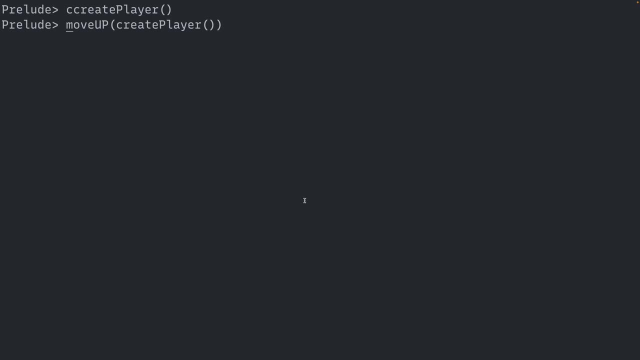 This seems like terrible code to just wrap them in parentheses and parentheses and parentheses And plus functions don't have side effects. And think about what that means. They can't modify anything outside. By displaying a number on your screen, you're modifying the pixels on your screen. 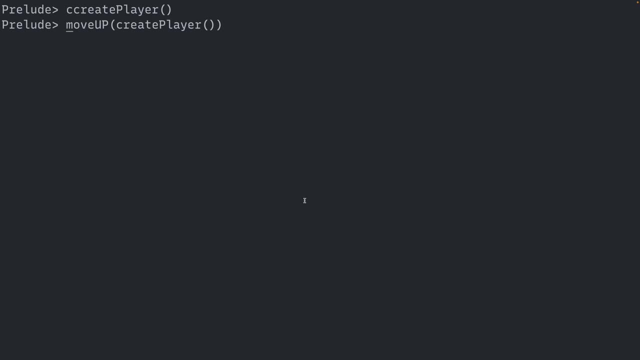 therefore modifying the information that goes into your eyes, therefore modifying the information in your brain, et cetera. That's not allowed in Haskell. So the answer to this situation is that you cannot have all pure functions, because then you can't have any input or output. 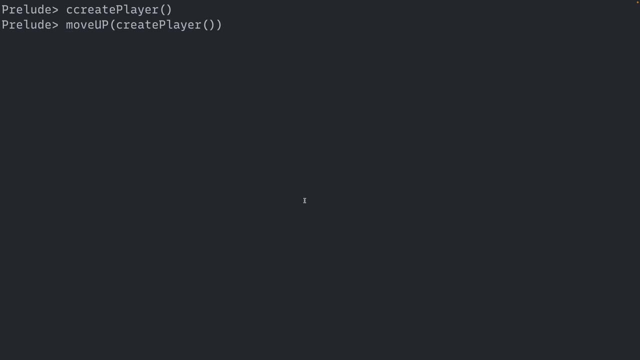 So the solution is the creation of a new type called io, which all functions that interact with the outside world must return. Therefore, functions that don't accept this type are not able to be used along with these functions, because it will simply result in a type error. 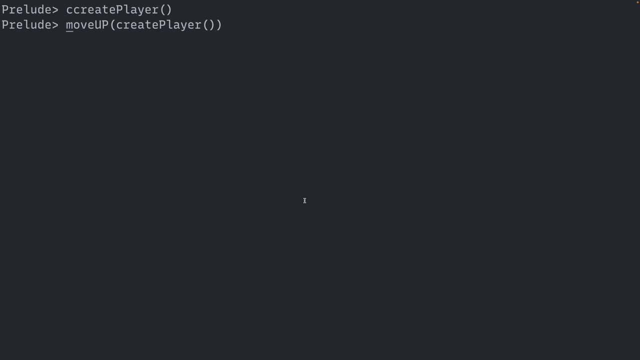 Now, using this method, it is able to be separated out from all of the pure functions. But before we get into that, let's take a brief detour into the complicated subject of monads. Okay, let us actually look at something a bit more theoretically. 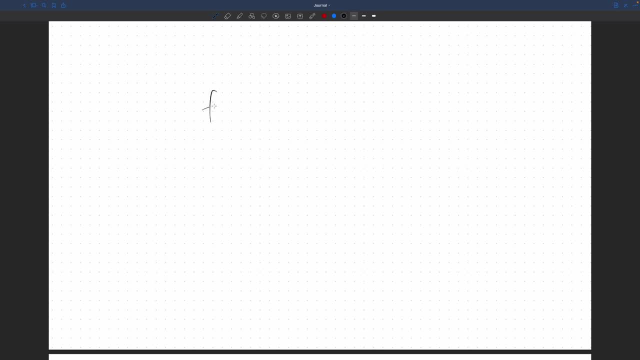 and just the logic of how stuff works. So, first of all, if you have a function that relies on the output of another function, so you pass one into the other- you can also write it in a way that basically makes it easier to read. 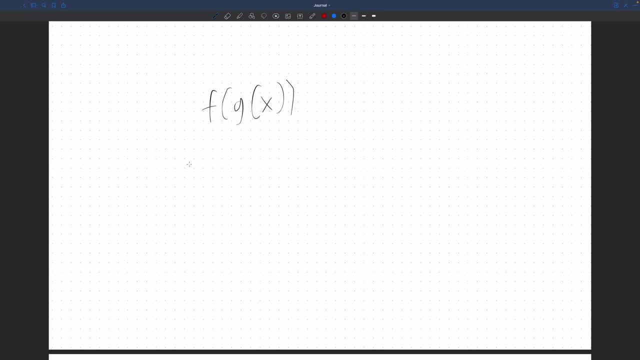 Instead of one inside the other, you can just say like one to the value of the other, So you can write something like g and then to f and then to something else. Or you can rather say x to g, basically just passing values around to each one function to another function. 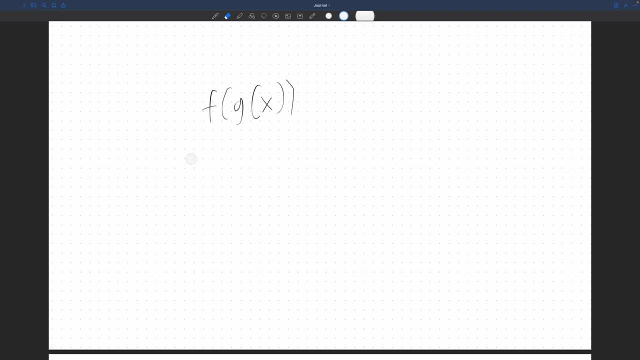 And I'm just going to use this syntax- and in Haskell there's actually an operator that kind of does the same thing and we can talk. if you want, you can look into that further. So for types, of course you can have stuff like numbers. 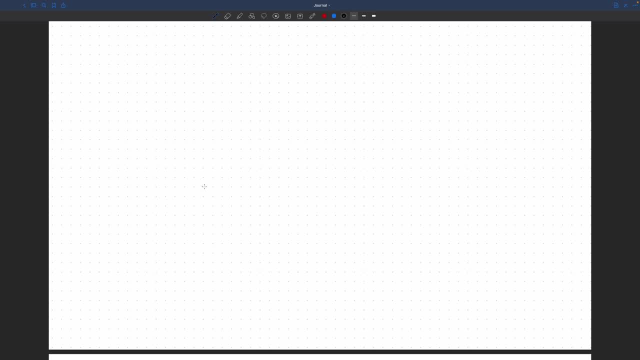 you can have strings and everything else. So let's say we are making like a linked list or if you don't know what that is, just think of like a bunch of trains. Maybe the trains have a property. that's like train, like the carprevious right. 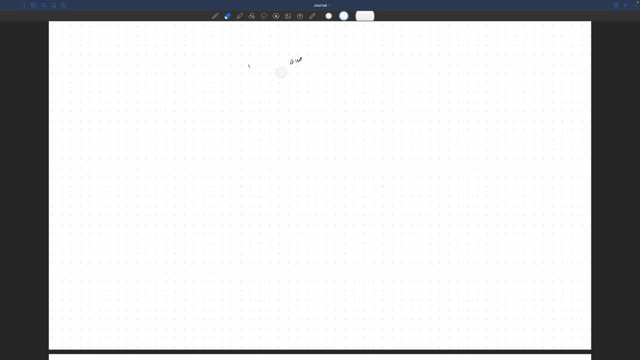 So it will give you the previous segment or the next one, But sometimes it might be nothing if it's just a list, What in most languages would be something like no, or undefined or something like that, but Haskell doesn't. So here's where we introduce the type: maybe. 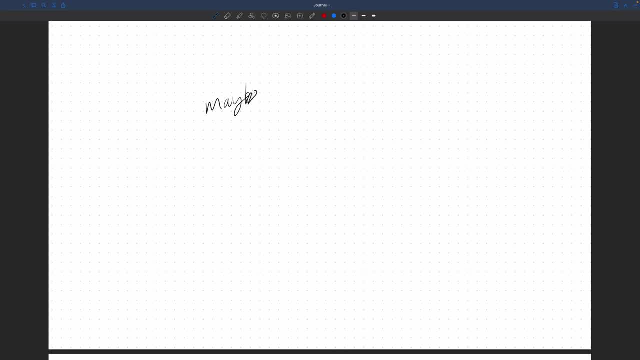 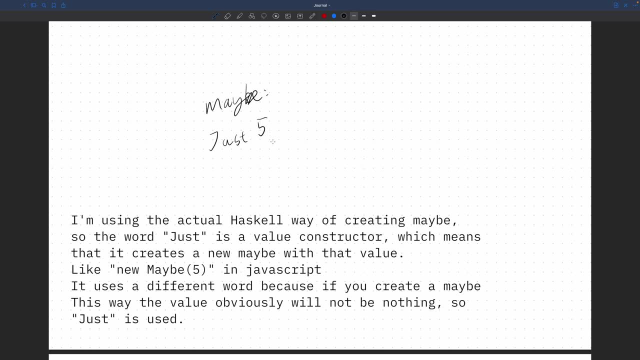 So for maybe right, for maybe you can have two types. It could be just, for example, just the number, Let's say we're dealing with numbers. It could be just five, or it could also be nothing. That's the two types it could have. 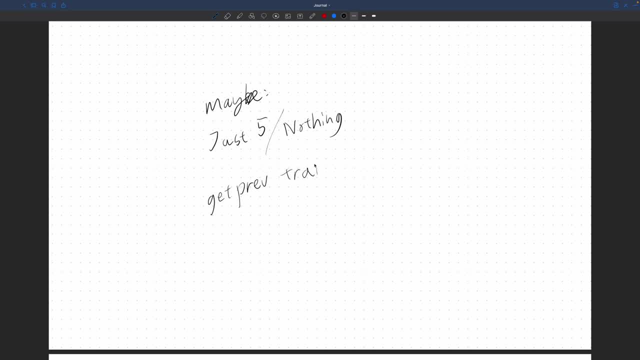 You can write a function like getPrieve and then you need to pass it in like the current car or the current train and then it will return you like, for example, either just the train or nothing, if it doesn't exist. 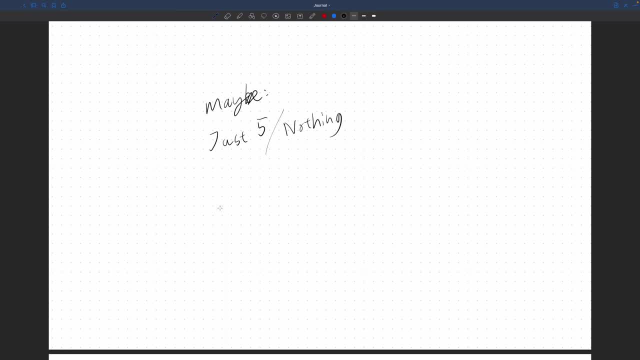 That's very simple. But maybe you want to get it twice, Maybe you want to get two segments above. Well, how do you do that? Like a logical way of thinking about it would be like: get you know, getPrevious, getPrevious right. 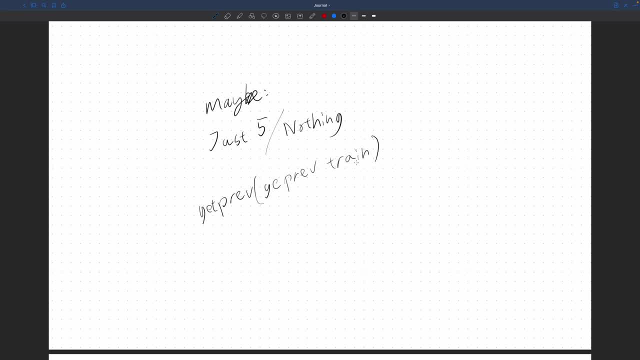 getPrevious, getPrevious in the train. But this wouldn't work, And maybe you can see why. maybe you can't Because the reason is that the train, the input to getPrevious, is simply train right, The input to getPrevious, you simply give it a train. 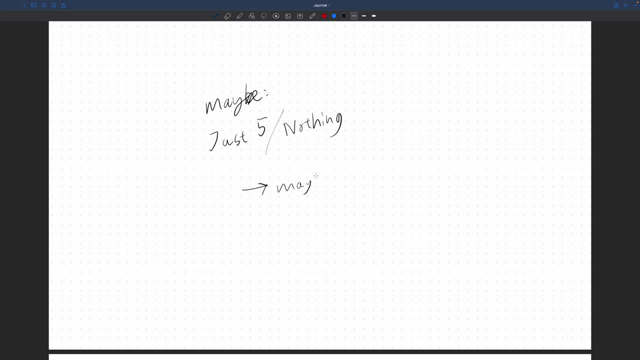 But the return output is maybe, And it's maybe train, something like that. And here's the problem. You can't pass maybe train as the input. It has to be 100%. You know where it is. So now we are right on the problem. 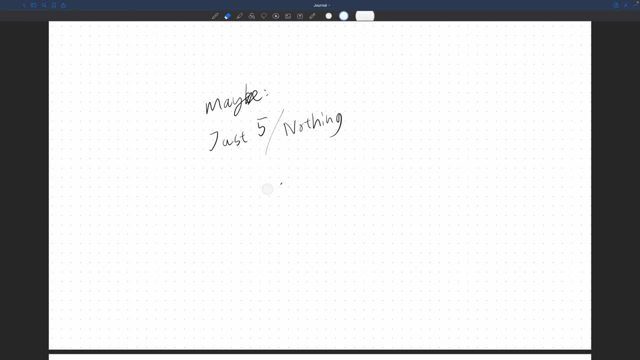 But like one way to solve. it would be like we use something called case or like if statement. It's like if it is actually a value, if it is actually calculated, or else if it's nothing, just simply do nothing again, And this works. 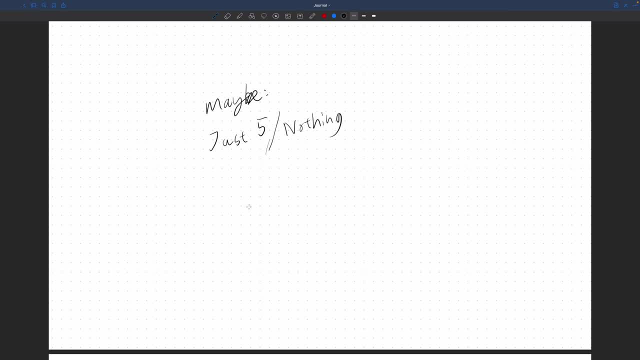 But you can see how it becomes really tedious if you were to have multiple functions that you just want to simply chain together. however you can. And now, where's like our clever part about? basically, monads come in. So, monad, all it does is like a special operator. 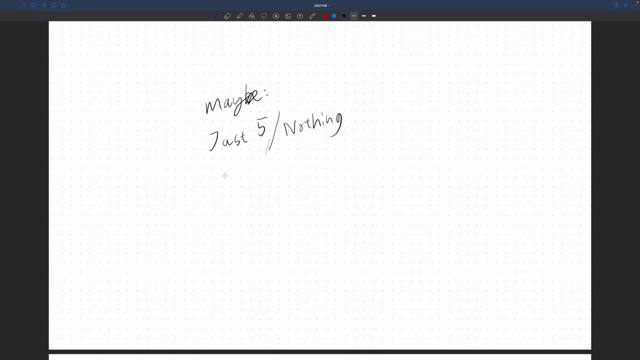 So, instead of passing your value directly into the function, you pass both the function and your value into another function that deals with how it's supposed to be done, like how its value is supposed to be given to the fed into the function. So for maybe we can write our custom function. 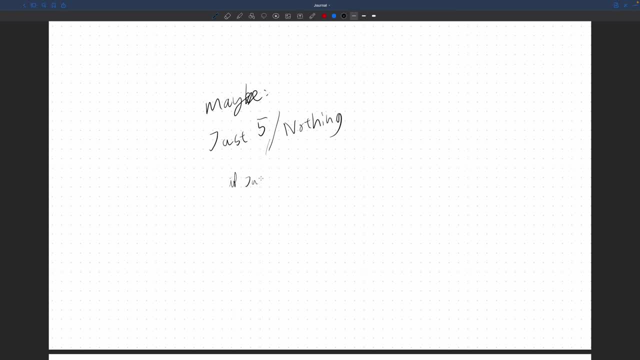 That's very simple. We can just like say if it is like just like x, then just say like, call it like fx, like that, Or like maybe like else, just like you know return nothing. or just say like else is nothing. Of course this is in Haskell. 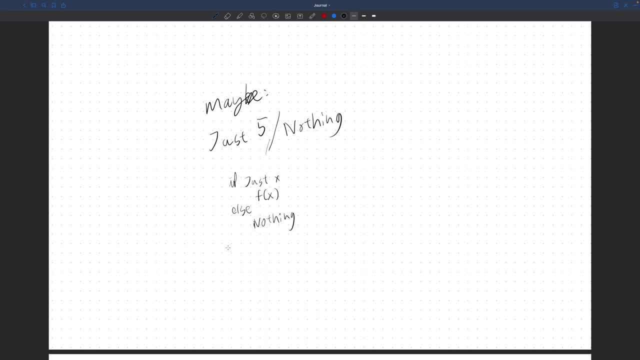 You can't run this, but just as an example, And this basically does what it does. This is what we want. So let's say, we define it as using like something like a double arrow, right, So we can just simply now say: train. 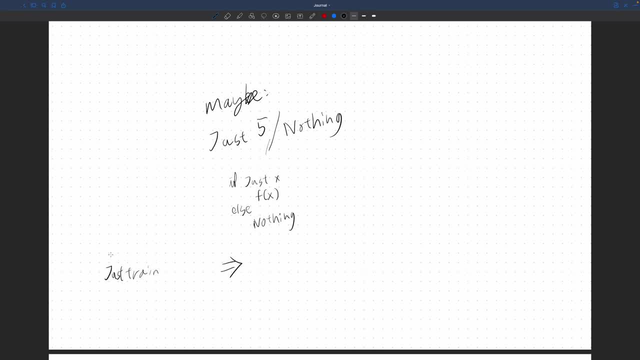 But we had to create it as before, as just the function, right, We had to make it into the type, So it has to be just train like or simply as train into, And then we can give it a value to that function. So like: get previous right. 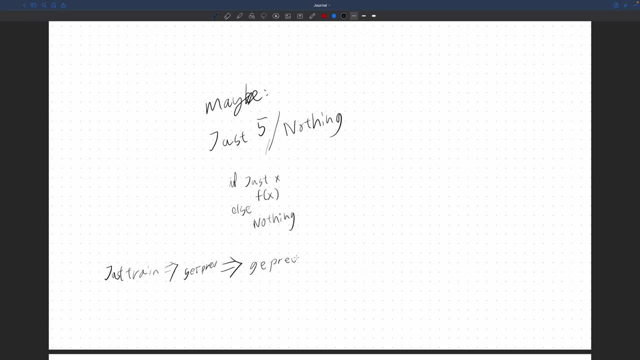 Prev, get previous, And this essentially does what we want, because it takes just train and just separates out the value here and passes it into this, which represents the maybe, And then we just simply separate that out again and pass it into that, Or if it's nothing, we can simply basically skip it and simply return nothing. 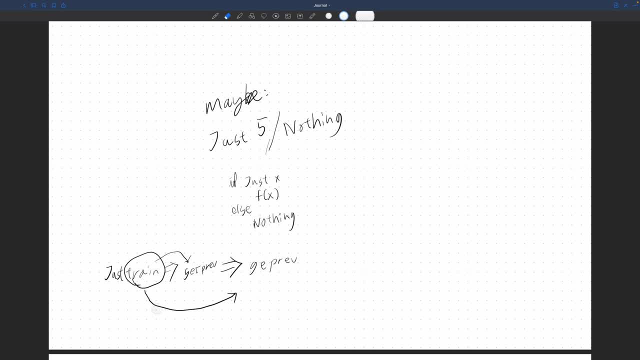 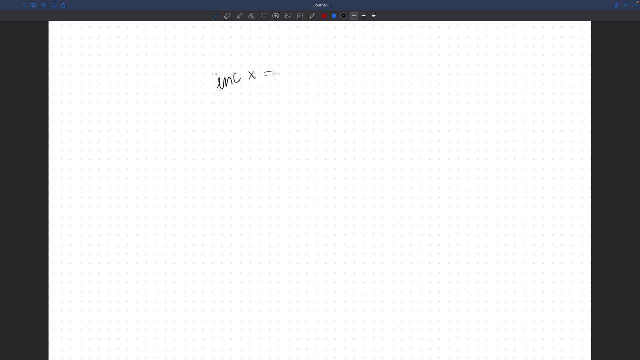 which you can go into this function and chain together however you would want. So just to give an example, Just to give an example of another monad, maybe we can say: we give a function called increase which increases x and basically just gives it x plus 1.. 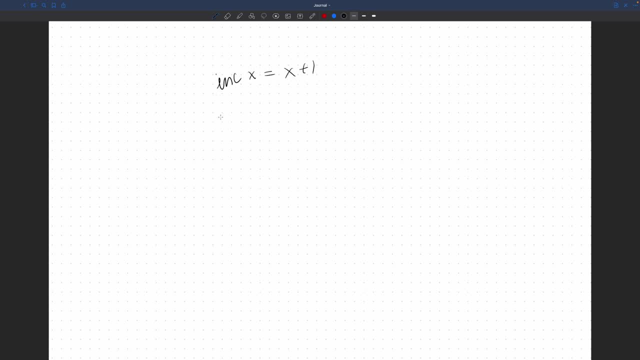 But, however, like we cannot use consolelog in this world, So what if we say something like that simply just passes another string along as a log result. So we can just say: maybe we can say: increase x. We can use something called a tuple, which is like a pair of values. 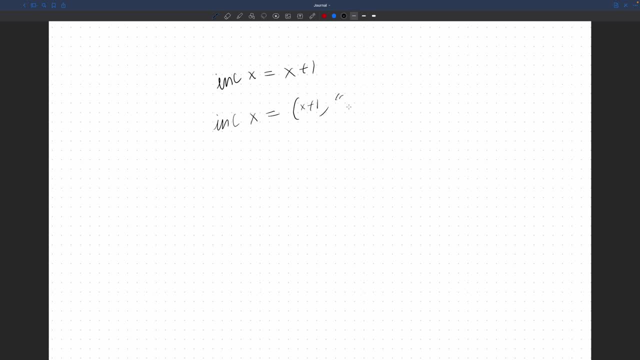 We can say: the first value is your actual result, But the second value is like maybe, like wow, big number, or something like that, Right, Something like that. And just to standardize it, we can maybe call this tuple like a type of something, that's like log. 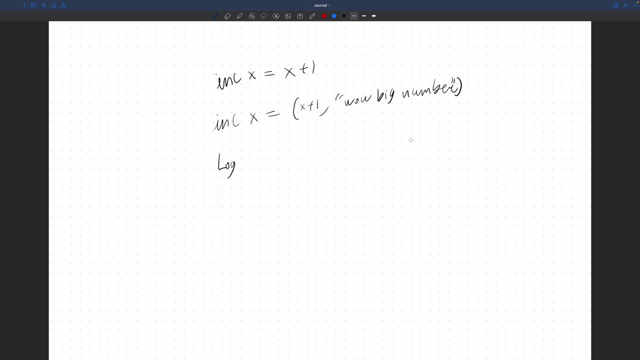 Right, You have the actual value and part and you have the log part. So now what you do? let's say you have another function called multiply, Or maybe like square. actually, just to keep it simple, have one function. Let's say we have a function called square x. 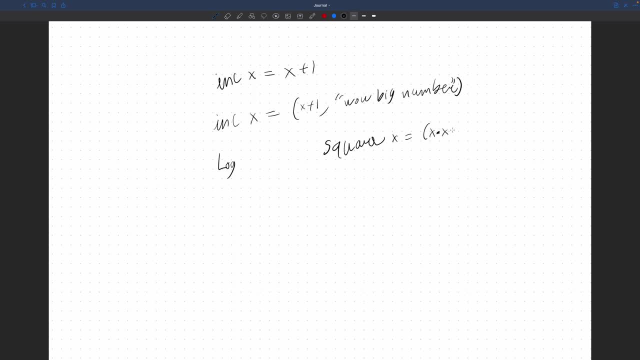 And it does the same thing x times x And then it has like hello or something as a log Right Say: you want that. But now we have the problem, Like, if we have 3, we want to make it so that you increase it by something. 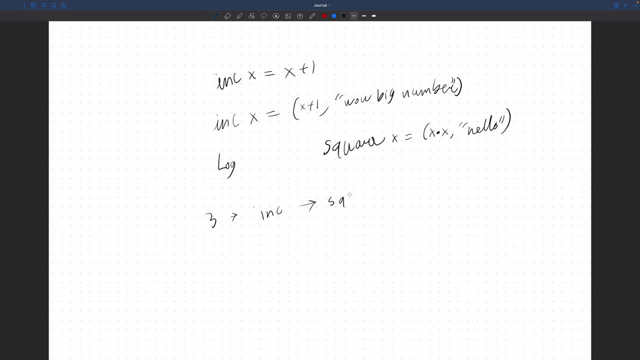 And then you square, So it's 4.. And then you square it, You get 16.. This, as we said before, this will not work because it wants a variable x, But you're actually passing in a tuple that has both x and hello. 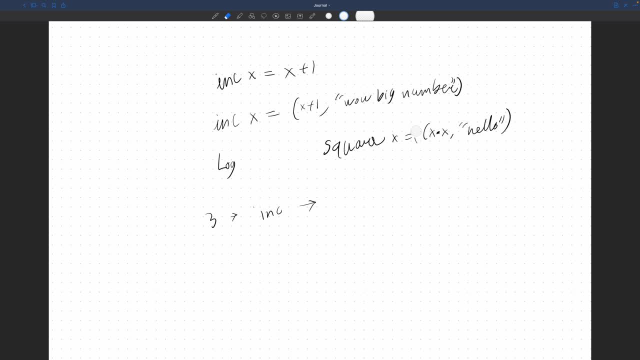 So of course you can rewrite your functions to do something that doesn't require this. You can rewrite your functions to maybe only take the front part. It's like x, zero is index or something, But that would be a hassle to do. 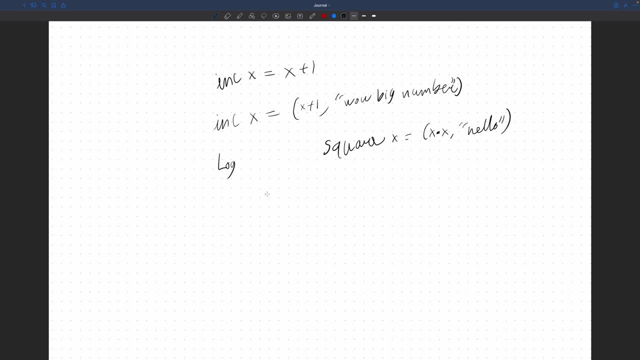 And it's quite annoying, Right? So now we can make a function that's like the arrow function be set equals to, like if it has f. Of course, I don't know why I use this notation. It might be confusing, It might be not. 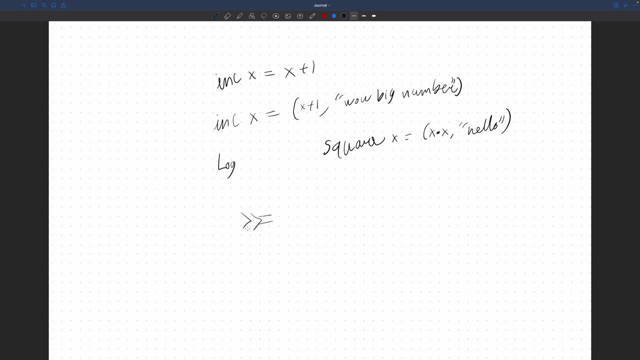 The actual notation is this: So bracket, bracket equals to: But the point is, what you can say is that you take the value right, You take the log, which has both the value and the text, and you separate it out. So you separate this thing and you. 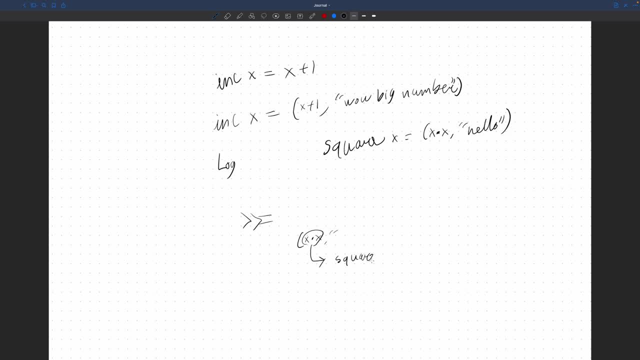 and then you actually pass it into the square function here And so you add back some message. So you have this part, or maybe you want to add the previous person's message as well. So now, with this message, you can pass along happily down the chain. 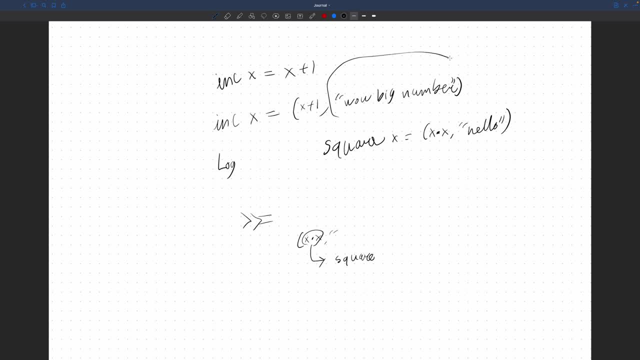 And you can say that we have here. we use the same for log just as like a comment. What we can also do is emulate state by having a variable that gets passed along all of the expressions but it just maintains the same value, or you can optionally choose to change it or differentiate with it. 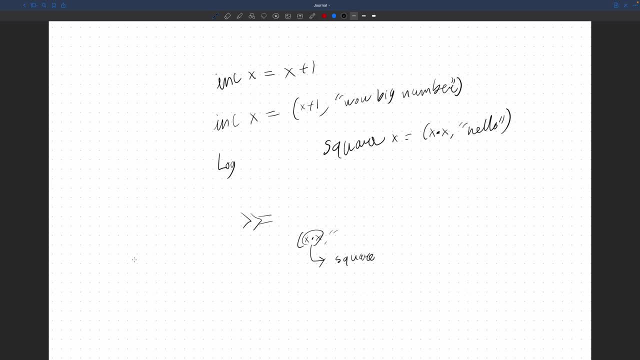 You can see that we can start from value, We can change it, We can choose to mutate it however we want. Okay, So now we turn back to the real problem of reading and writing user input. So these functions are what we will use. 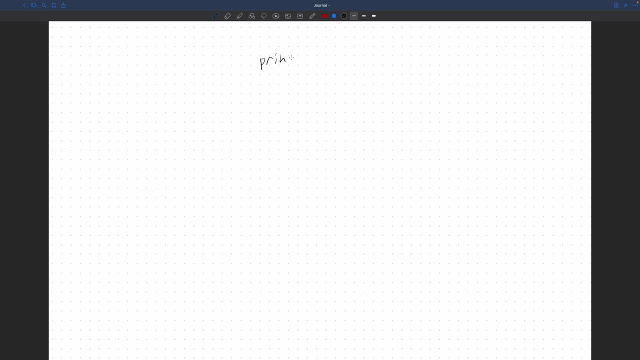 We will obviously call on here. So there's, I'm just going to impure. So I'm just going to first tell you that there is a function called print and there's a function called get line. Print just prints a value. 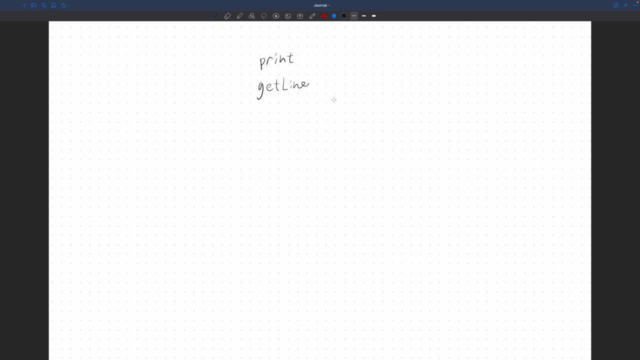 get line simply gets a line that's inputted from the user. So let's see how this is done Basically. as I have said, Haskell, you cannot try to, for example, pass in a function that express expects an int. 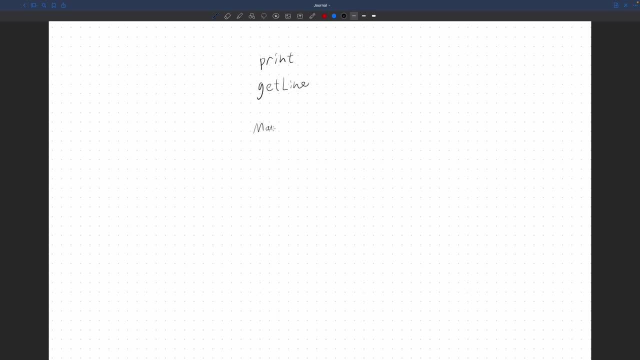 a string that will just immediately file. And also with the maybe thing. you cannot pass in something that is part of a maybe like wrapper, when the function is simply expecting the int value. So the creative thing is that, instead of get line being something that returns a string, 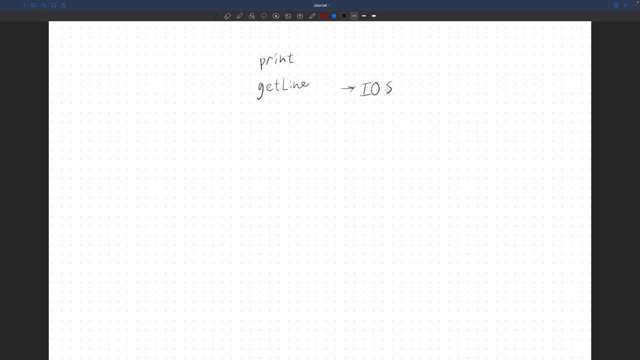 it actually returns a new type called IO string, And what this does is that if you try to pass it in, for example, let's say, use our count method, right, If you say count get line, this will fail. It will say something like expected type string. 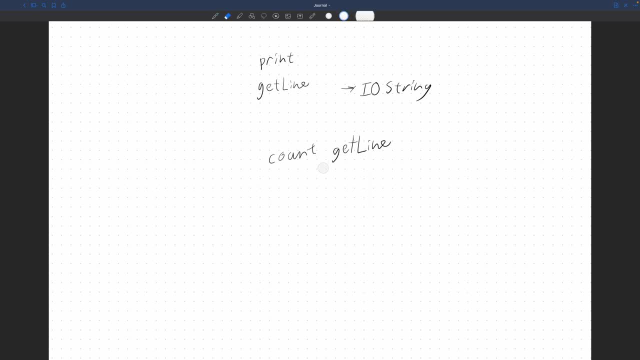 but instead got IO string so that you cannot mix and match these. And this highly encourages facts of using pure functions, that only using these to get them separating out so that your logic is very easy to organize. But you might think what's the point of writing normal functions? 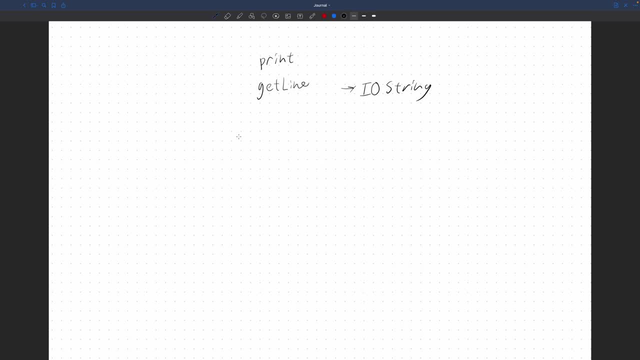 And if they can't interact with each other, don't you have to write all functions to accept the IO string, And that's where the monads come along. So you have, you can start with a function that's like get line right. 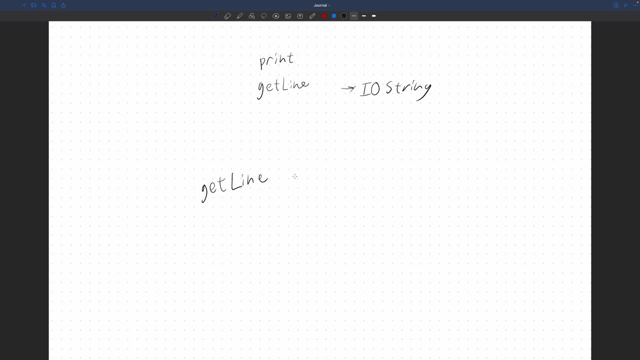 And I'm not going to use the arrow thing because that's misleading, I'm going to use the actual thing, which is this: right, Get line, That value gets passed into a function, Let's say count, And this does exactly as we said before. 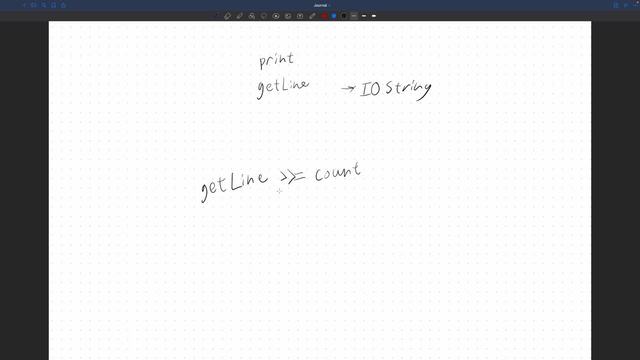 you can implement a custom method for each of these monads and say: define that. in this case, what this arrow does is basically take the IO out of the string and take out, take the inner inside value actually- and pass that into a count, because count expects a normal string. 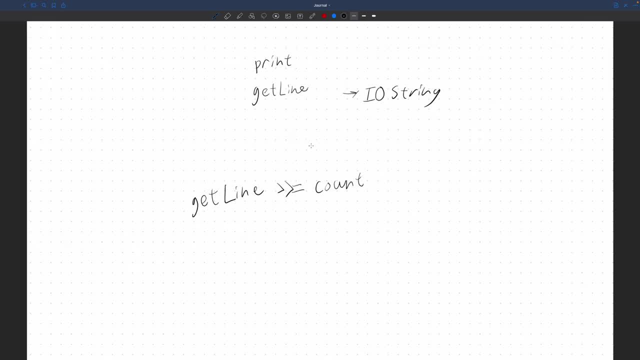 And that gives out your output. The fact that count returns to int isn't the problem. The problem is that the count function returns to normal int, not an IO int. So this means that for monads it's required that each of the steps have the same type on the outside. 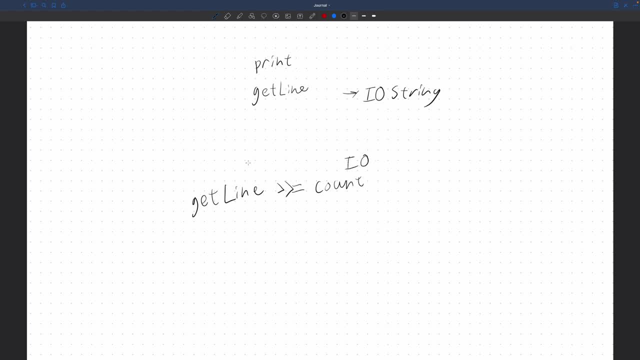 the same type IO, but it can change from, for example, an IO string into an IO int. That's perfectly acceptable If you want to do another operator and change this along. if it's an IO, then there's no point of doing this. 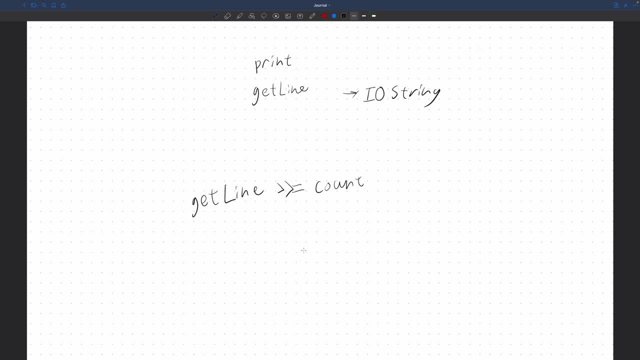 right To convert an int into an IO int. they offer a function called return And that's just a normal function. It's not a keyword. It's very misleading due to the name of it, But all it does is that if you give it an int, 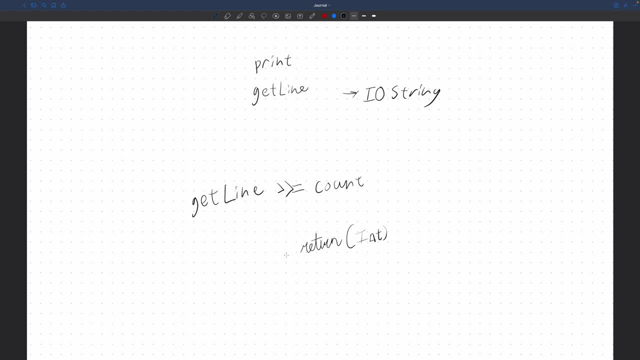 and also the outside context of this is that we're using IO. then it simply changes int into an IO int. That's all it does. But we can't exactly wrap it around. count like this, return count, because we still had to pass in the variable. 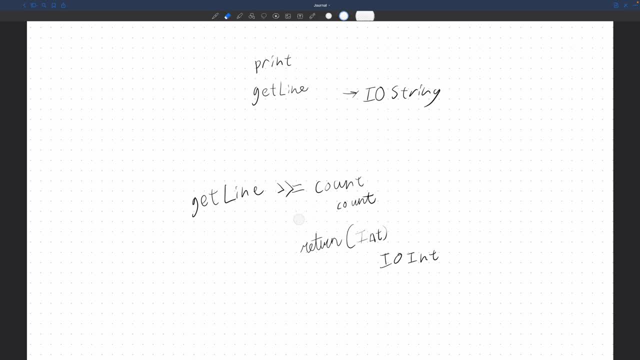 the value here into count. So we can't just return it directly, because that would be just returning the count function. So it won't be IO int, but simply IO of string function. It's going to be like a function which is like, not correct. 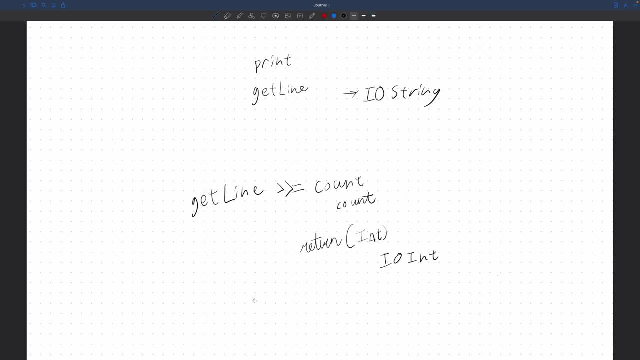 right. So to solve this problem, what we can do is write another helper function That's like combine right. Do that? First of all you have the first F and then you have a second function And then you have the actual value here. 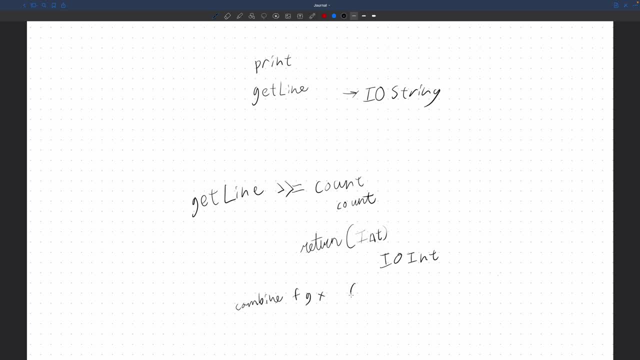 So what you can do is call essentially F of G of X, like that. This is of course also not real class code, just to make this a little bit easier sounding. And then what we can do here is basically write instead of count. 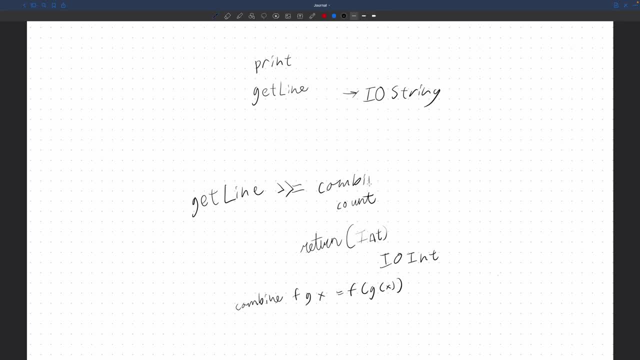 we write combine, Combine, return and count, And we can omit the X because of partial functions, So you can simply: this would itself would be a function that works in this case, And actually we don't need to write our own function this time, because Haskell. 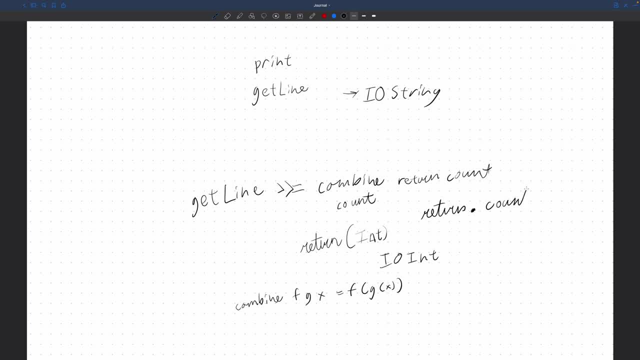 because we use it so often. this is a default. We simply write return dot count with a space in between, because this is actually a function just uses special name And it does exactly the same thing as combine, except we write it in the middle. 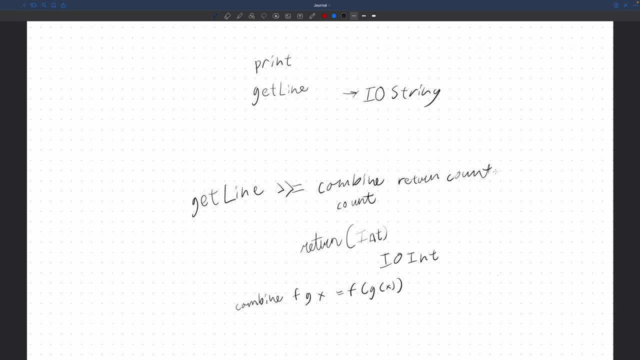 But now we have that. What we can do is: now it returns the IO int. We can- maybe we want to print it right. What we can do is just add another one. We just change this along And then we write: print right here. 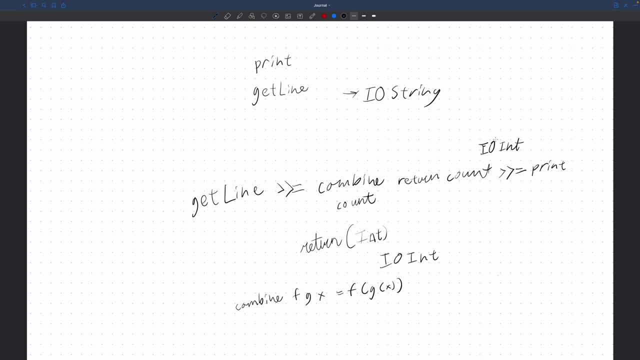 Because the IO int- int accepts a regular value, So it takes int, puts it into print and print actually returns the IO. nothing written like this right. Two parentheses mean nothing because print doesn't need a value to be returned, but it still has the IO property. 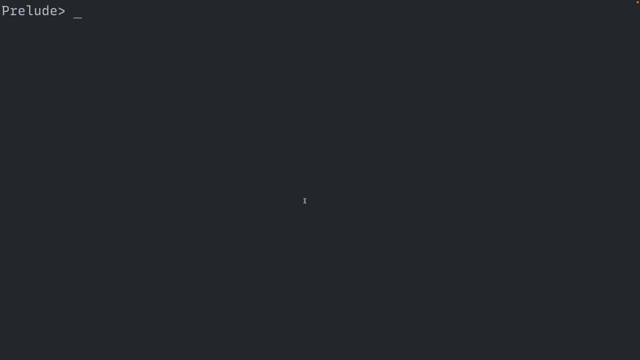 And that could be our end of the expression. Okay, so let's look at the function get line. So you can call it just simply like this, without no parentheses, And you can say hello and it will give you the string hello. But let's check the type. 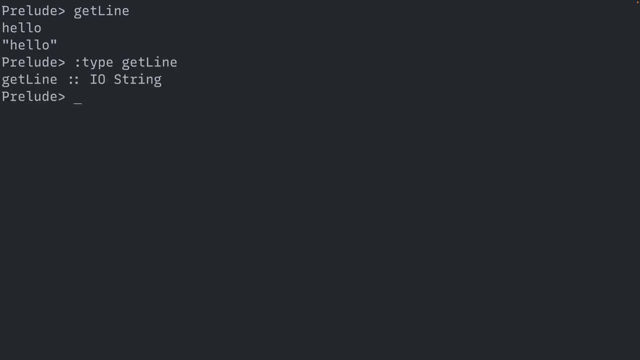 Let's check the type of get line And you can see it's an IO string. For example, if we had our original count function, it would give you an error like expected string, but got IO string. Now let's look at another function: print. 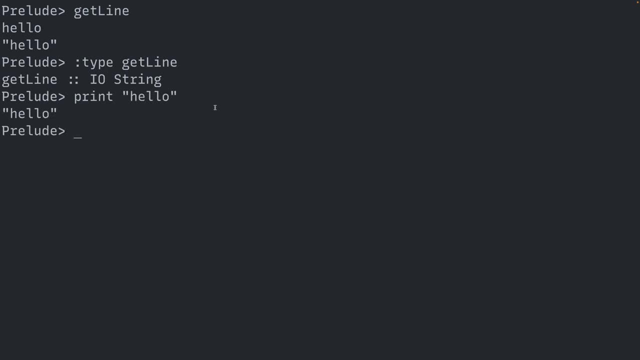 And print does what you expect. Print hello gives you hello, So we have print. Let's check the type of print. Type print: It says you have show a, but basically it's like anything that could be shown, So it's not just a string. 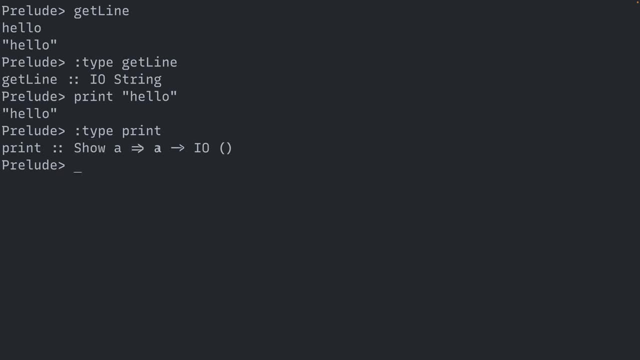 but we can ignore this and basically say: it's a string, It's an IO, Nothing. This doesn't mean like you're calling IO or anything. This just simply means nothing because, like print, doesn't return a value of any type. Cool. 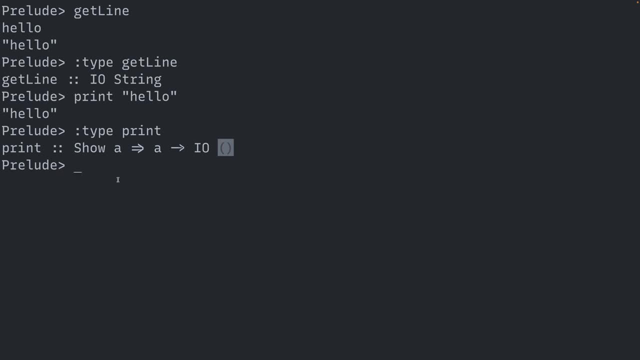 However, we can't say print, get line, as you might have expected, because it's expecting a normal value. So what you can actually do is use that operator I was talking about and then you say print. So now you can say: well, 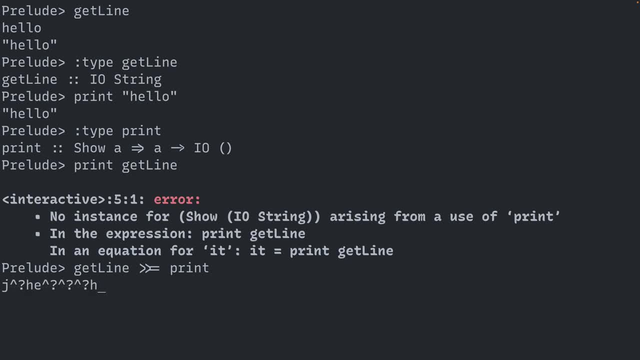 you can't delete, but you can say this, and then it will just give you the value. So that's it, And then it will just give you that. And if you're confused on what's happening, basically you're taking the IO string. 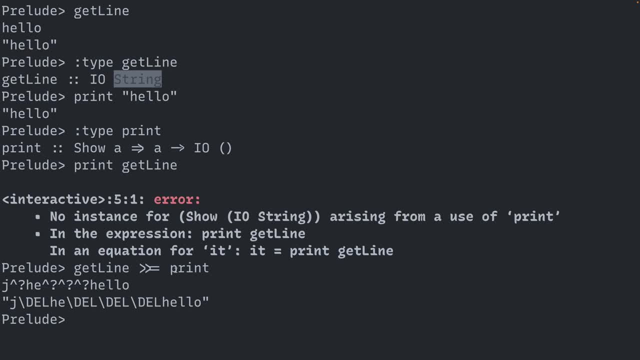 you are ripping the string value out of it, You're passing that into print, which can print that, and then prints it out, And so you can type kind of like: pass this back out a lot, because this returns the IO string, So that's a valid return value.